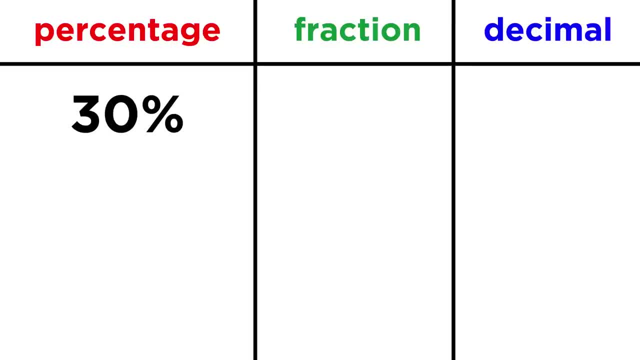 Let's take something like thirty percent. It's very easy to convert this to a fraction, because we know that percentages are out of a hundred. so thirty percent becomes thirty one hundredths or thirty out of a hundred. Then to reduce the fraction, we can divide both numbers by ten, and here's a hot tip. 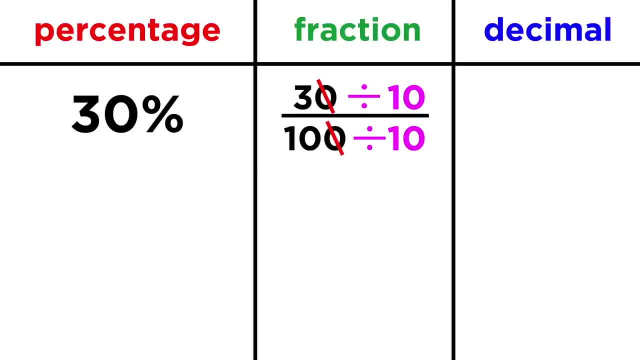 when we do this, we can just cross out the zero in each number, as that will do the same thing as dividing by ten. That leaves us with three tenths. So thirty percent is a fraction. It's equivalent to three tenths. 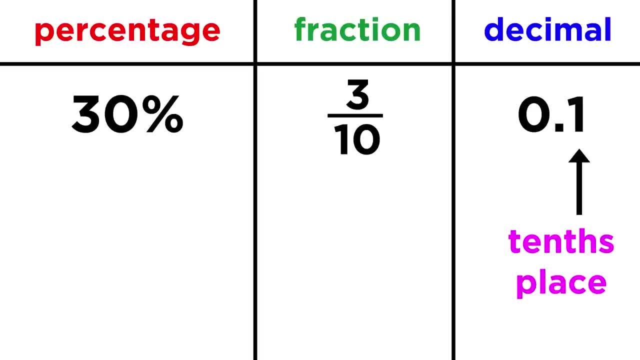 Now let's get that as a decimal. Well, we know where the tenths place is. so if we have three tenths, we just need to place a three in the tenths place. so zero point three, And there we have three different ways of expressing the same value. 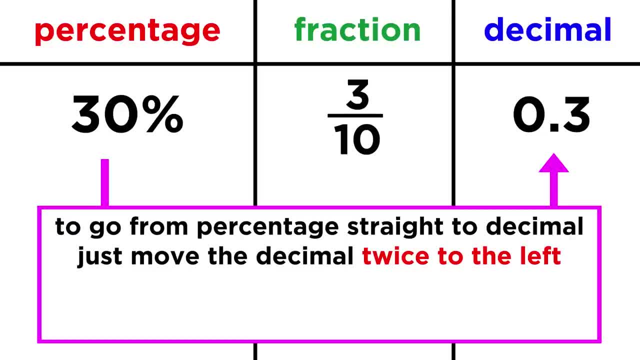 Here's another hot tip: when converting from percentages directly to decimals, all we have to do is move the decimal place twice to the left, Because one hundred is two orders of magnitude greater than one. So from thirty percent we just take the decimal place, which isn't written but is implied. 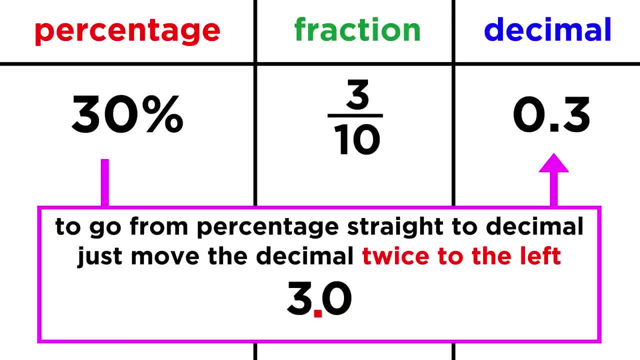 to be just to the right of the units place and move it over twice to the left. We can never start a number with a decimal point. there has to be a zero first. so that gives us zero point three. We could do the same with an eight point two. five percent sales tax. we move it once and 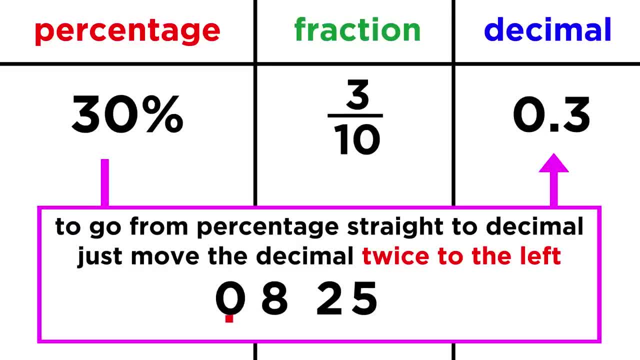 then if we have to move it again but there are no more numbers, just put a zero And there we have zero point zero, eight, two, five or the sales tax expressed as a decimal. This is useful because if you want to compute the sales tax on an item, you can just multiply. 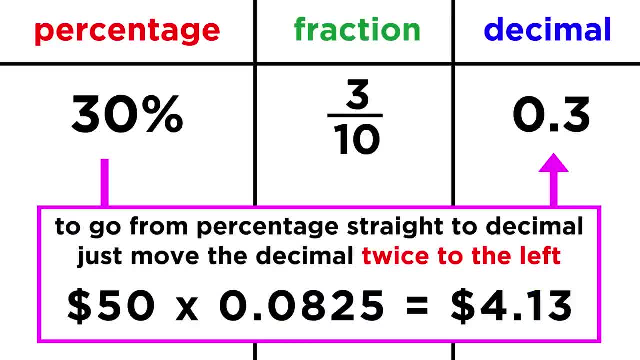 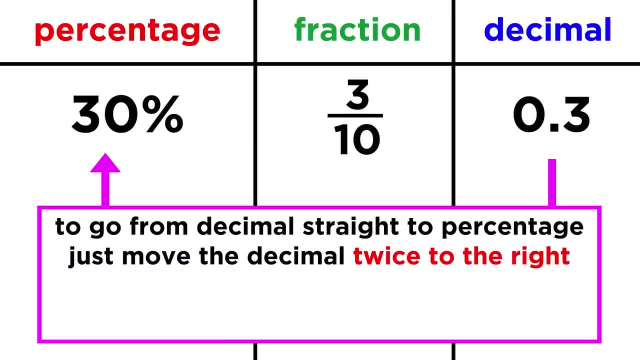 its price by this number. so a fifty dollar shirt would have a sales tax of four dollars and thirteen cents. To go from a decimal to a percentage, We just move the decimal twice to the right, because this is the same thing as multiplying by a hundred. 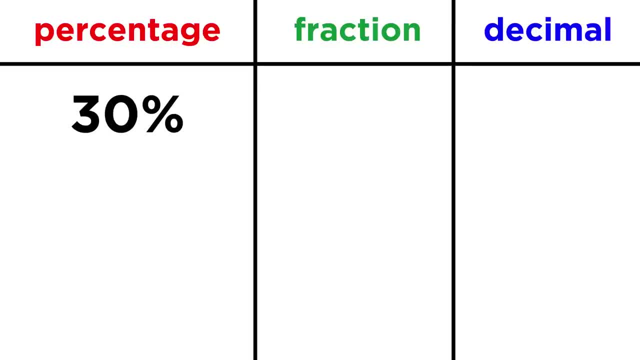 Let's take something like thirty percent. It's very easy to convert this to a fraction, because we know that percentages are out of a hundred. so thirty percent becomes thirty one hundredths or thirty out of a hundred. Then to reduce the fraction, we can divide both numbers by ten, and here's a hot tip. 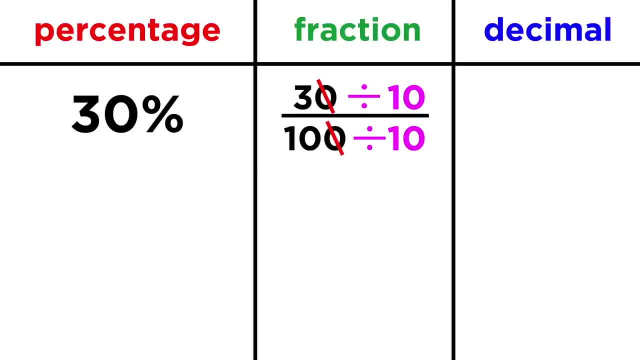 when we do this, we can just cross out the zero in each number, as that will do the same thing as dividing by ten. That leaves us with three tenths. So thirty percent is a fraction. It's equivalent to three tenths. 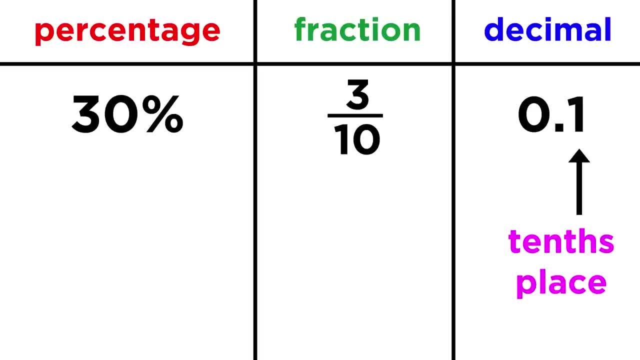 Now let's get that as a decimal. Well, we know where the tenths place is. so if we have three tenths, we just need to place a three in the tenths place. so zero point three, And there we have three different ways of expressing the same value. 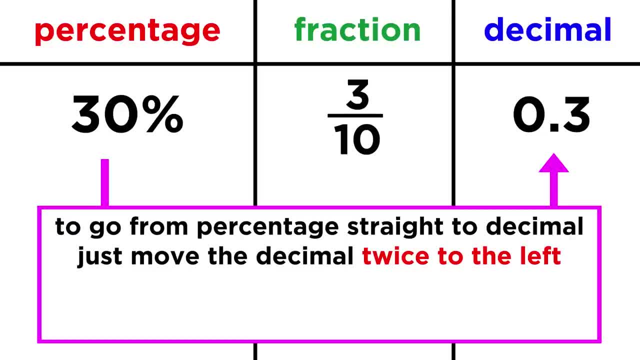 Here's another hot tip: when converting from percentages directly to decimals, all we have to do is move the decimal place twice to the left, Because one hundred is two orders of magnitude greater than one. So from thirty percent we just take the decimal place, which isn't written but is implied. 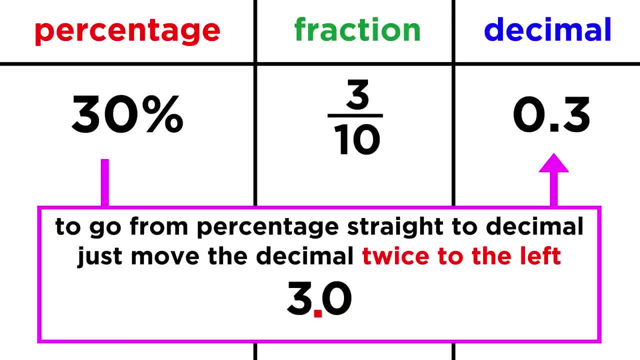 to be just to the right of the units place and move it over twice to the left. We can never start a number with a decimal point. there has to be a zero first. so that gives us zero point three. We could do the same with an eight point two. five percent sales tax. we move it once and 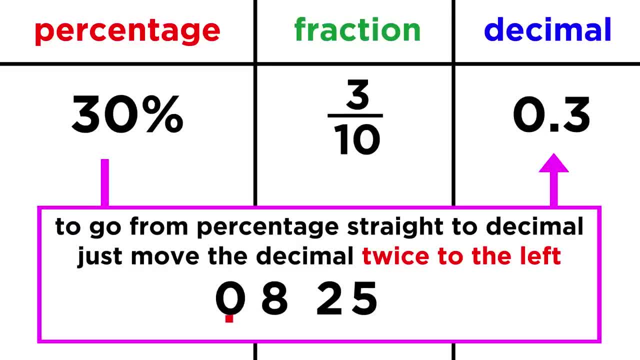 then if we have to move it again but there are no more numbers, just put a zero And there we have zero point zero, eight, two, five or the sales tax expressed as a decimal. This is useful because if you want to compute the sales tax on an item, you can just multiply. 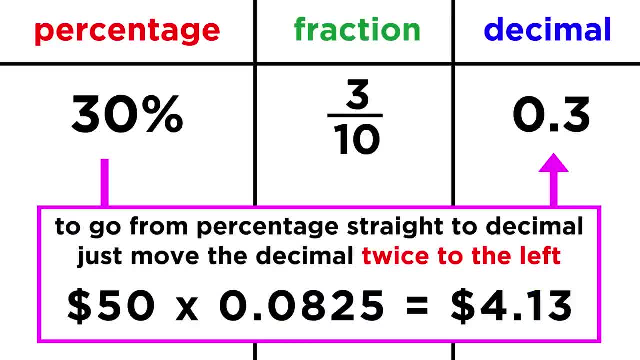 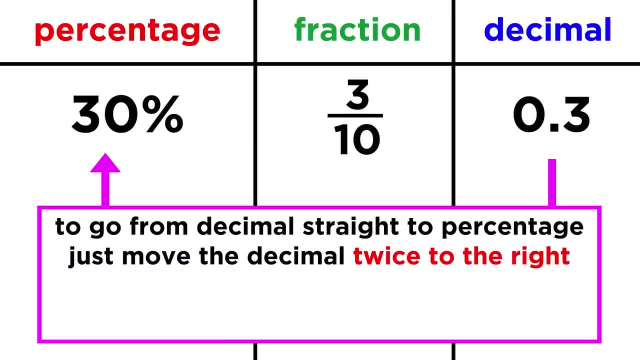 its price by this number. so a fifty dollar shirt would have a sales tax of four dollars and thirteen cents. To go from a decimal to a percentage, We just move the decimal twice to the right, because this is the same thing as multiplying by a hundred. 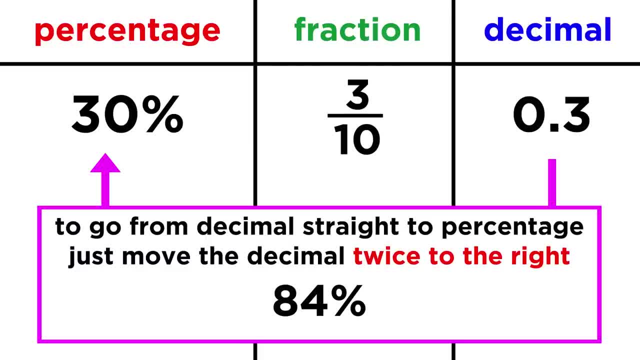 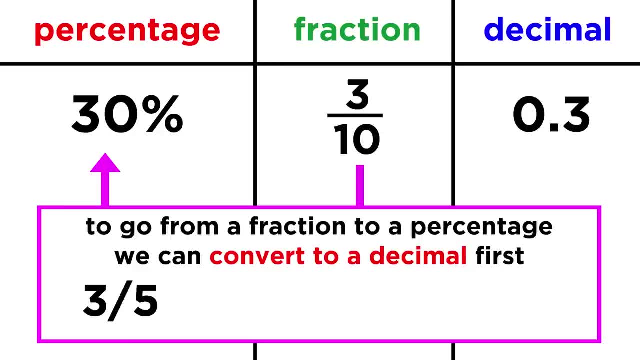 So zero point eight. four becomes eighty four percent, To go from a fraction to a percent. we could convert the fraction into a decimal first, For three fifths. first we can ask what is one fifth as a decimal? That would be zero point two, because five of these or five fifths would add up to. 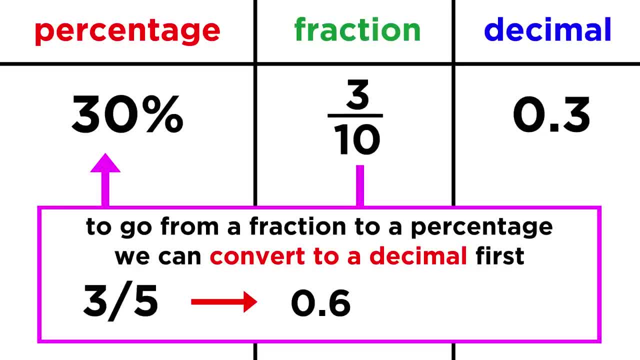 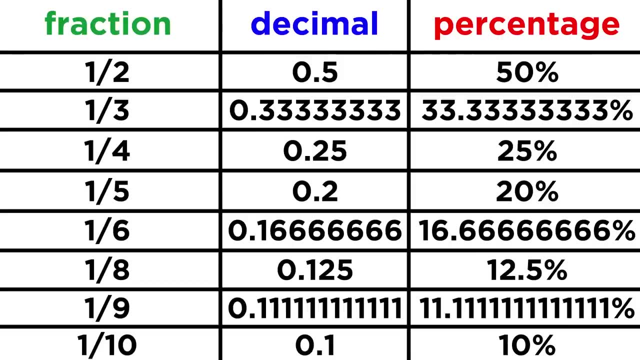 one. Three fifths must be zero point six. From there we just move the decimal over twice, adding a zero, since we need to, and we get sixty percent. Here is a table with some common fractions and their corresponding values as decimals and percentages. 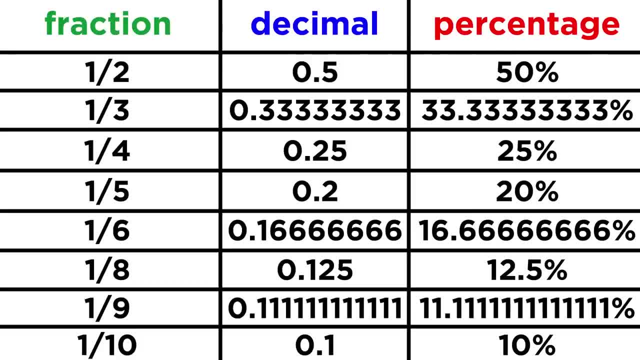 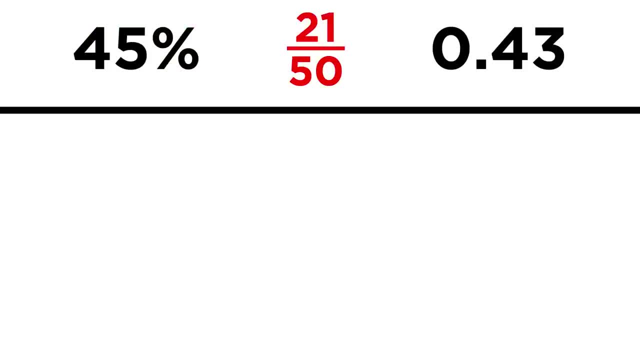 We should be able to convert between these forms with ease, as these are all just different ways of communicating ideas that are useful in different scenarios. Let's try and put this to use. Here are three values: forty-five percent, twenty-one fiftieths and zero point four. 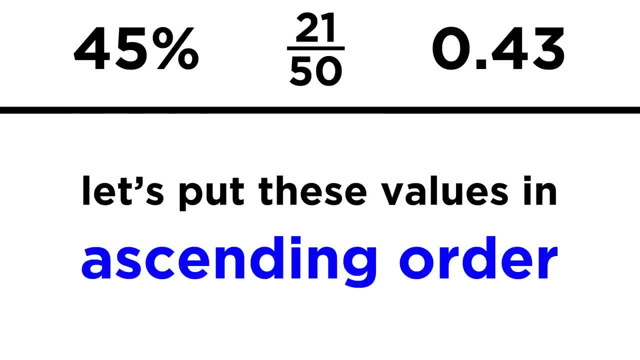 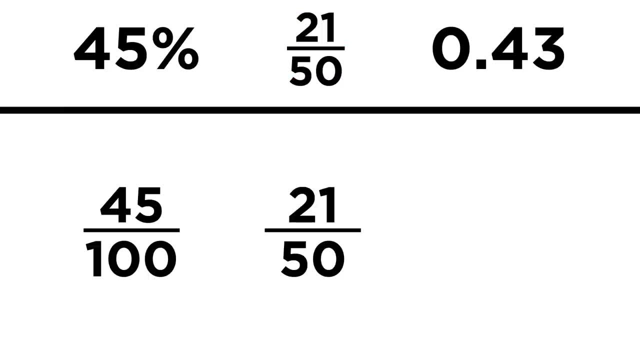 three. Let's try to arrange these from least to greatest. Well, forty-five percent is the same as forty-five over a hundred. What should we do with this fraction? Well, if we want to compare it to another fraction, it needs to have a hundred in the denominator. 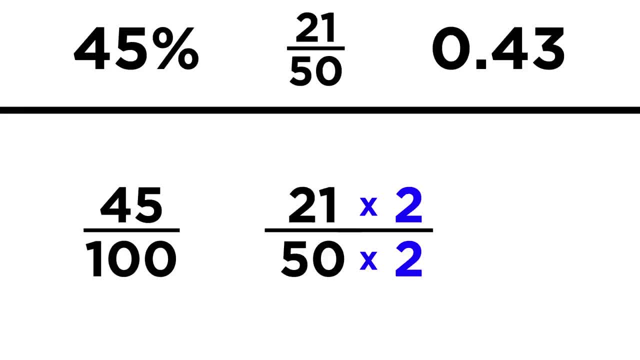 So let's get this one looking that way too. Multiplying both numbers by two, we get forty-two over a hundred, So we get forty-five over a hundred, So we get forty-five over a hundred, And with the final value, we can move the decimal over twice to get forty-three percent. 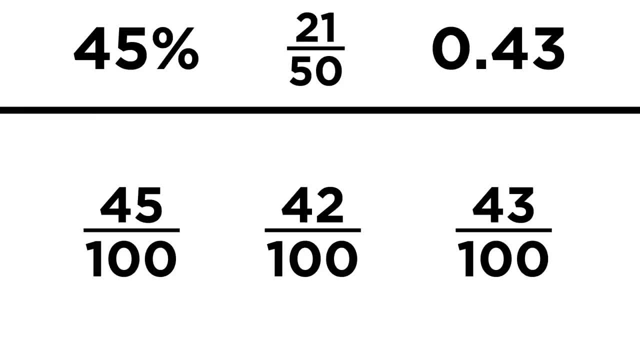 which must be forty-three over a hundred. Now it is quite easy to put them in order because they look the same: Forty-two comes first, then forty-three, then forty-five. That means that this will be the correct order for the original values. 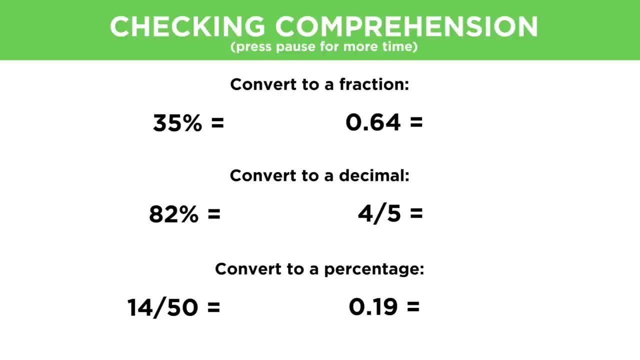 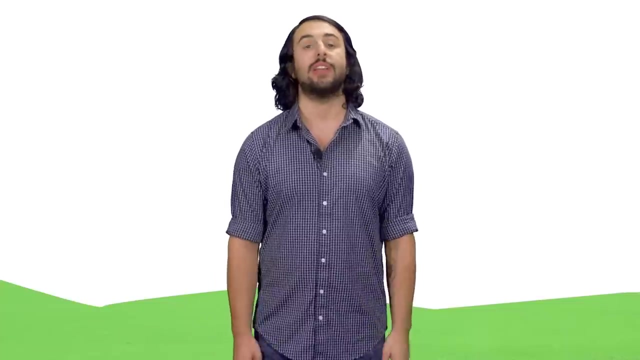 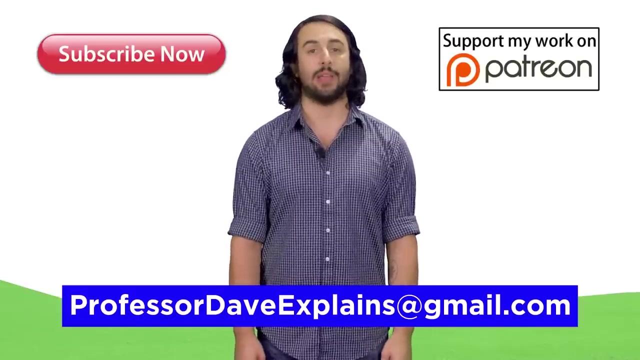 Let's check comprehension. Thanks for watching, guys. Subscribe to my channel for more tutorials. Support me on Patreon so I can keep making content and, as always, feel free to email me professordaveexplains at gmail dot com. 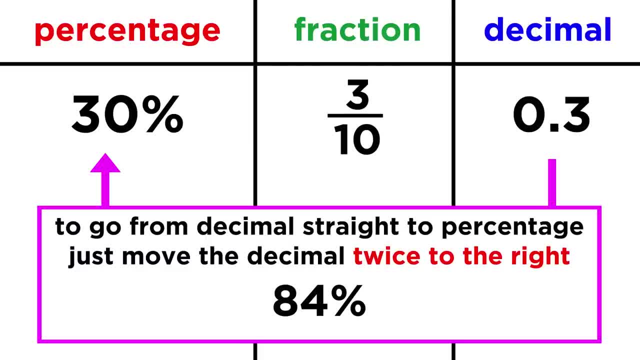 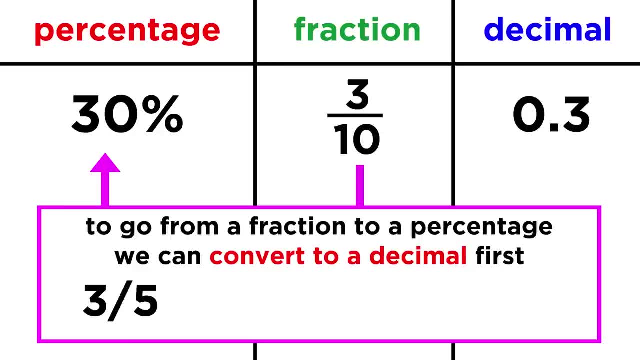 So zero point eight. four becomes eighty four percent, To go from a fraction to a percent. we could convert the fraction into a decimal first, For three fifths. first we can ask what is one fifth as a decimal? That would be zero point two, because five of these or five fifths would add up to. 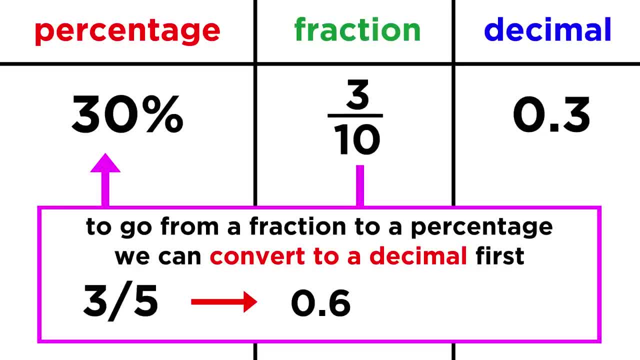 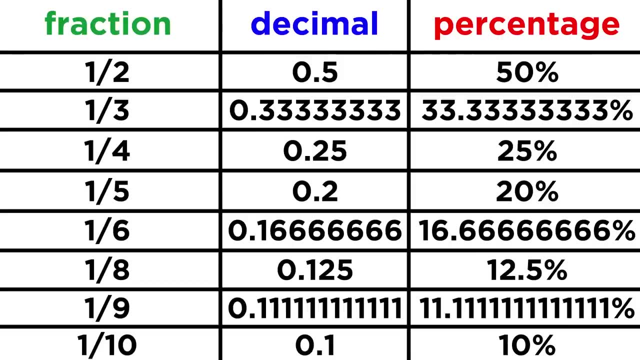 one. Three fifths must be zero point six. From there we just move the decimal over twice, adding a zero, since we need to, and we get sixty percent. Here is a table with some common fractions and their corresponding values as decimals and percentages. 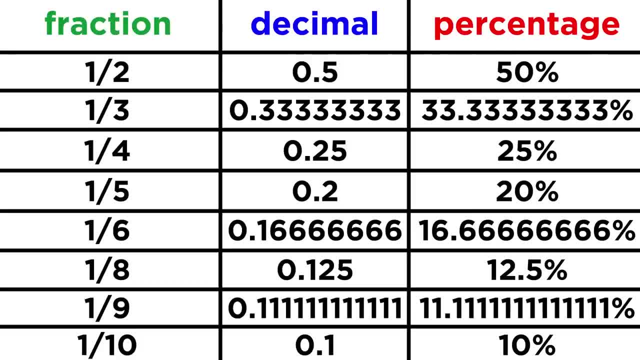 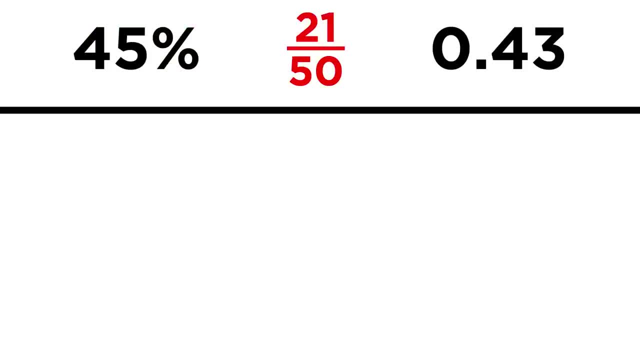 We should be able to convert between these forms with ease, as these are all just different ways of communicating ideas that are useful in different scenarios. Let's try and put this to use. Here are three values: forty-five percent, twenty-one fiftieths and zero point four. 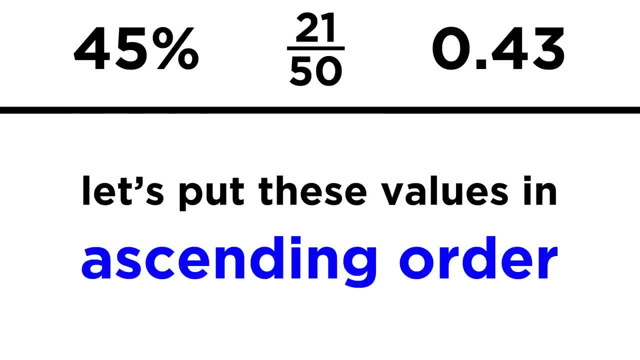 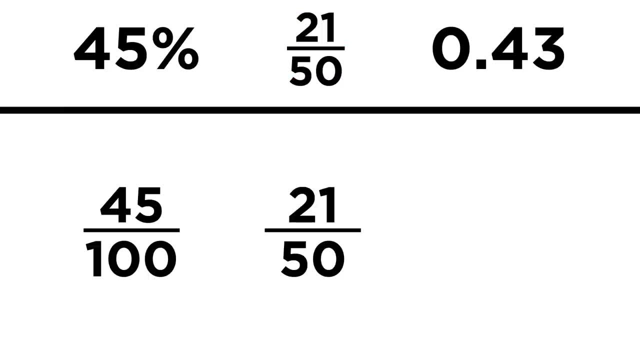 three. Let's try to arrange these from least to greatest. Well, forty-five percent is the same as forty-five over a hundred. What should we do with this fraction? Well, if we want to compare it to another fraction, it needs to have a hundred in the denominator. 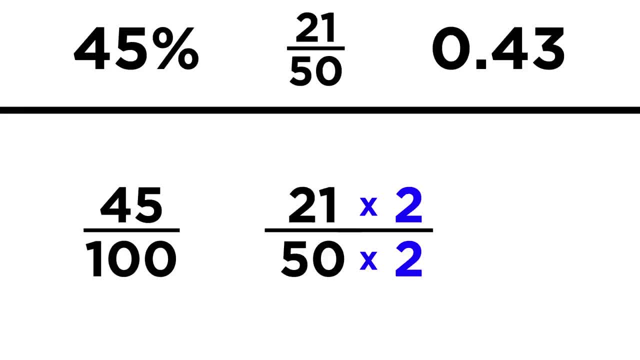 So let's get this one looking that way too. Multiplying both numbers by two, we get forty-two over a hundred, So we get forty-five over a hundred, So we get forty-five over a hundred, And with the final value, we can move the decimal over twice to get forty-three percent. 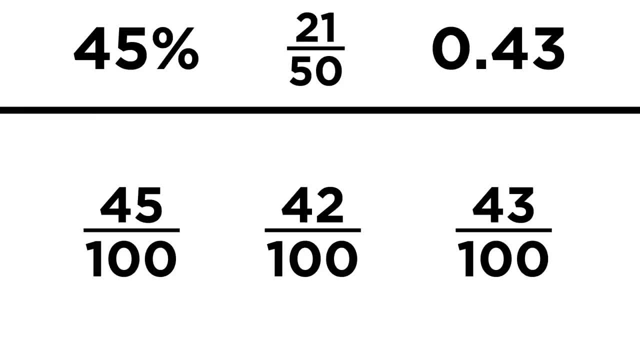 which must be forty-three over a hundred. Now it is quite easy to put them in order because they look the same: Forty-two comes first, then forty-three, then forty-five. That means that this will be the correct order for the original values. 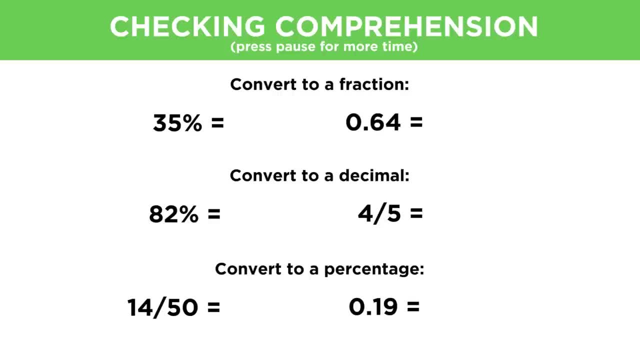 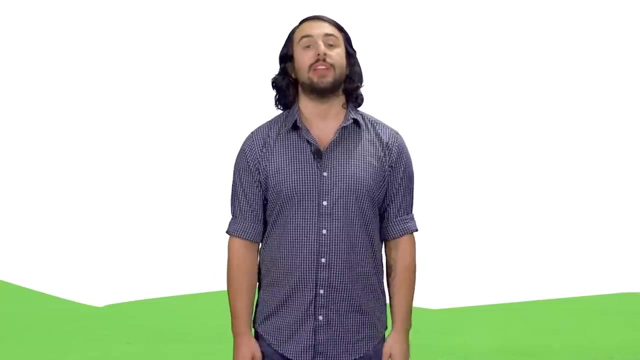 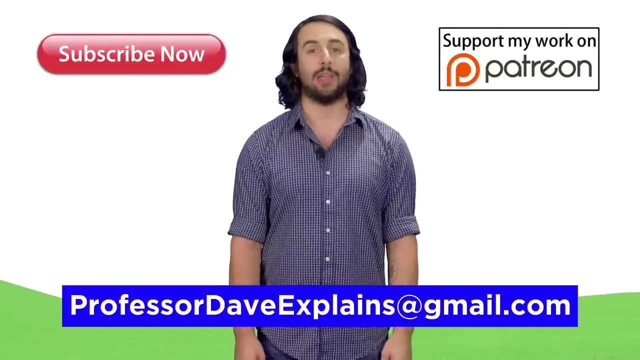 Let's check comprehension. Thanks for watching, guys. Subscribe to my channel for more tutorials. Support me on Patreon so I can keep making content And, as always, feel free to email me professordaveexplains at gmail dot com.